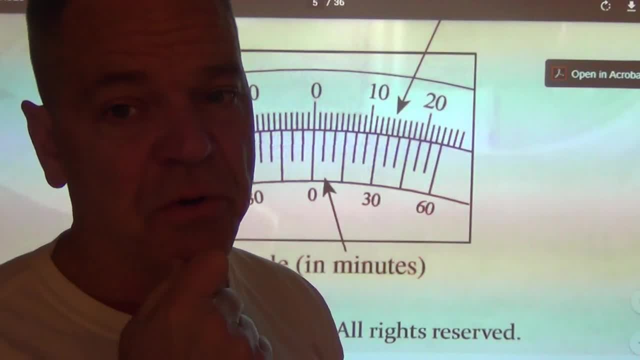 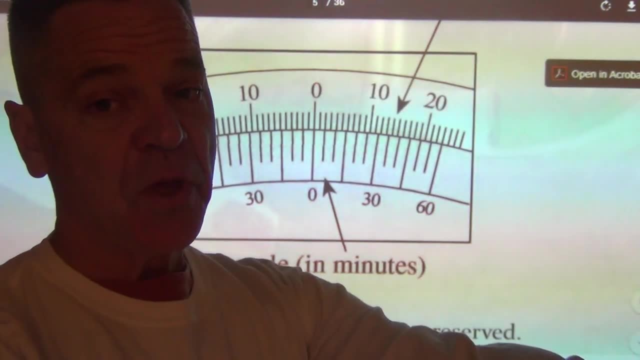 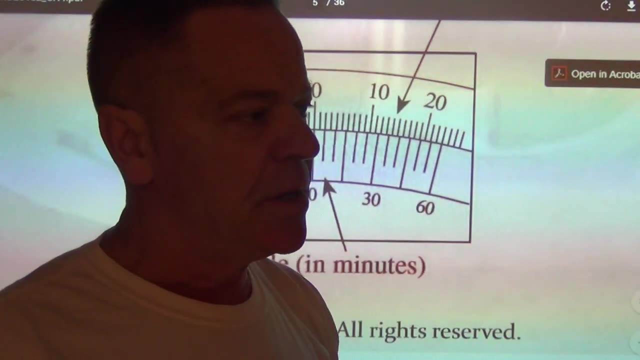 Okay. so I'm going to suggest to you a method here for constructing your vernier scale, right, for constructing a vernier scale on a protractor. And we have already done making a vernier scale on a linear scale. We've done a very simple version of that. but here's my suggestion. 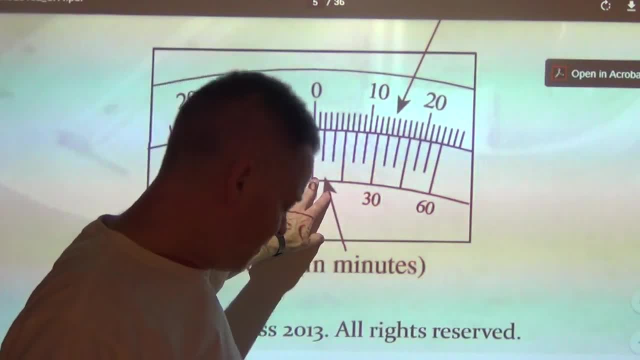 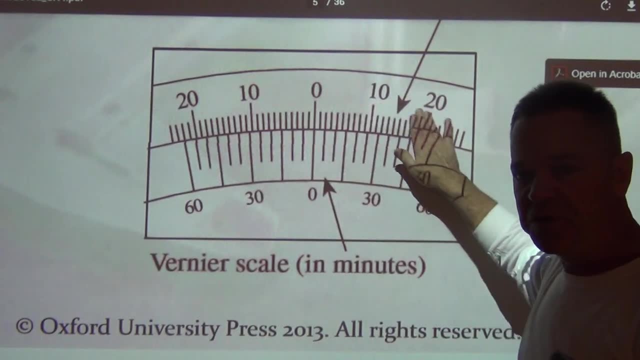 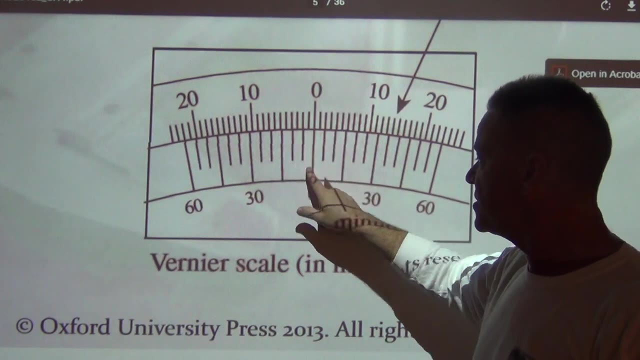 When you look at this vernier scale here, you can see that. And now, just to be clear, this is the main scale up here. These are whole degrees. Here's a zero mark And at the moment this is set with no fraction involved at all. right. 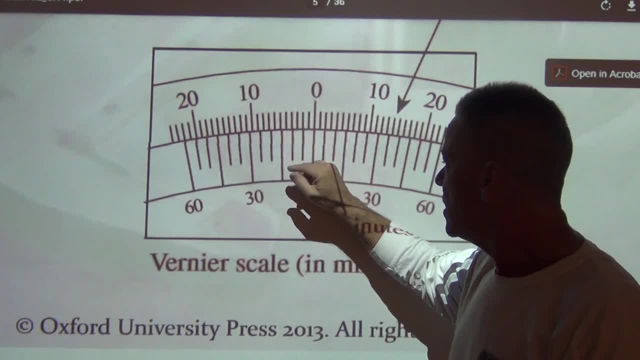 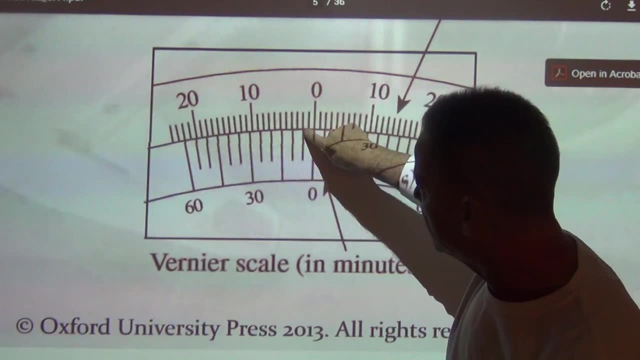 This zero lines up perfectly with this zero here, And when you look to either side you can see this lines a little to the left of the main scale line, This one's a little bit to the right of it, and so on. So this is centered pretty well. 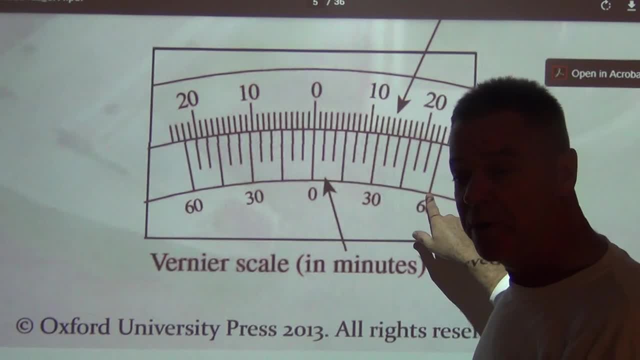 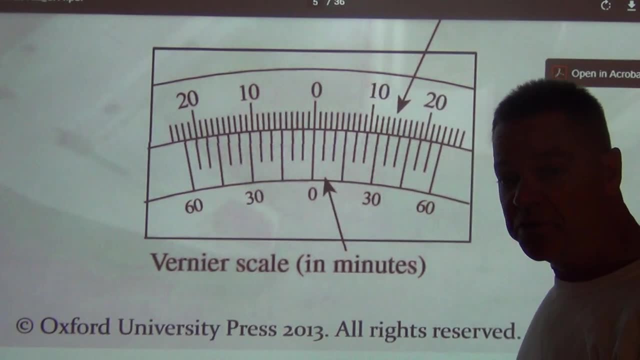 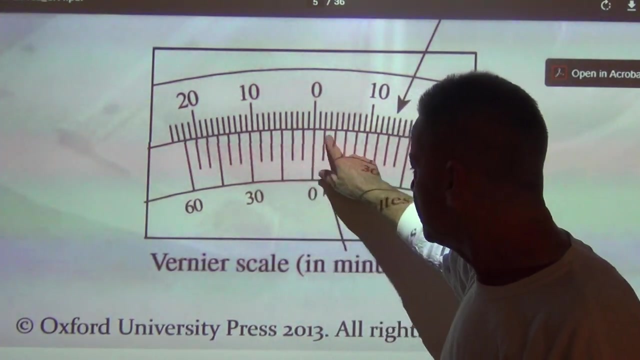 Now, when you go over here to this, The 60-degree mark, not surprisingly it lines up perfectly too right there on the main scale. Now here's my suggestion: If you look carefully at how this is aligned, this zero here, this zero lines up with the zero. 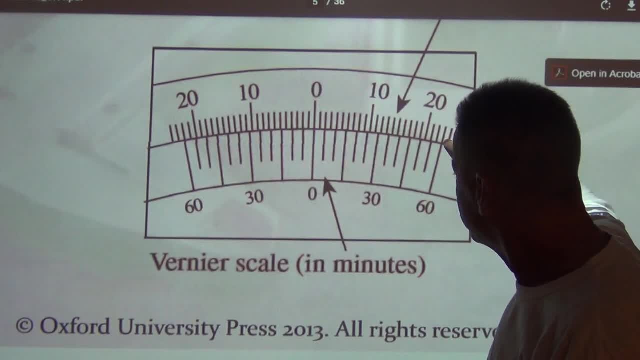 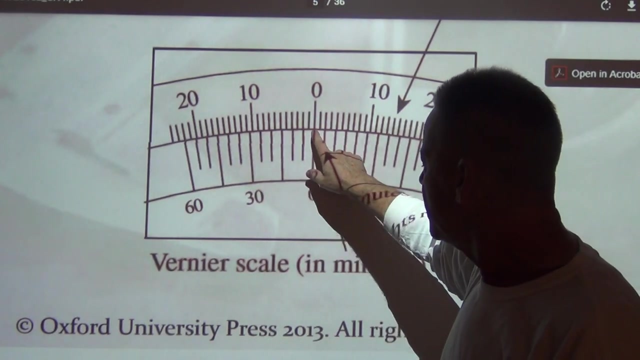 This 60 is over here at the 23-degree mark on the main scale. So to get from the zero to the 60 is 23 degrees on the main scale. So if you've constructed a main scale and you take that and divide, 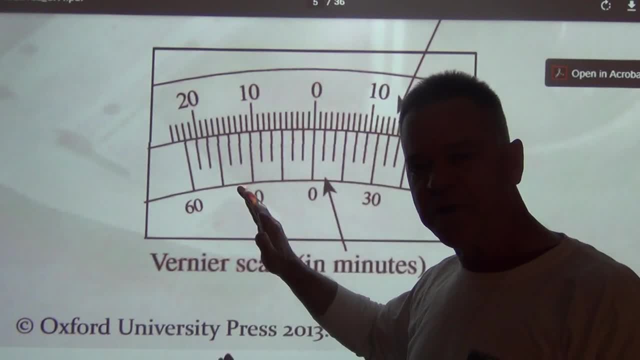 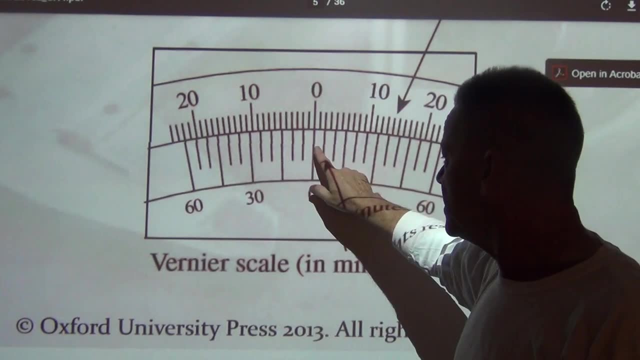 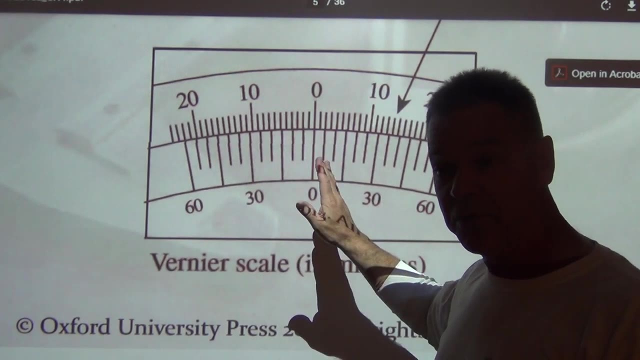 I'm sorry. You've constructed a main scale. You find the distance of zero to 23 degrees on the main scale and divide it up into equal parts- 12 equal parts. That's a little funky right, But I believe that will give you an accurate version of your scale. 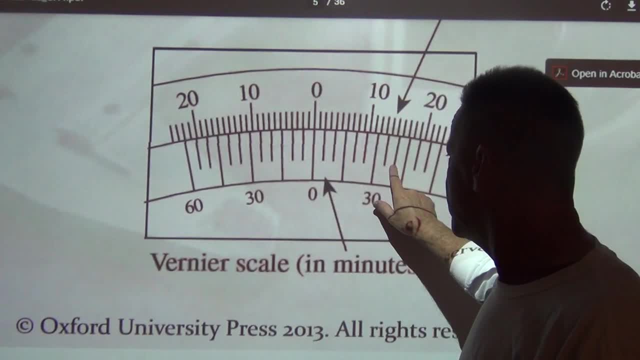 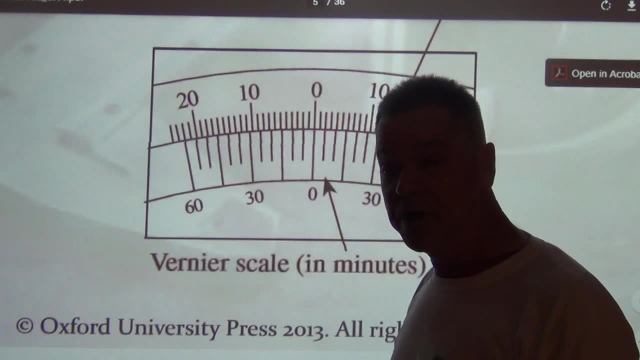 So this is 1,, 2,, 3,, 4,, 5,, 6,, 7,, 8,, 9,, 10.. 11, 12. Equal spaces here. They're not as big as a degree. 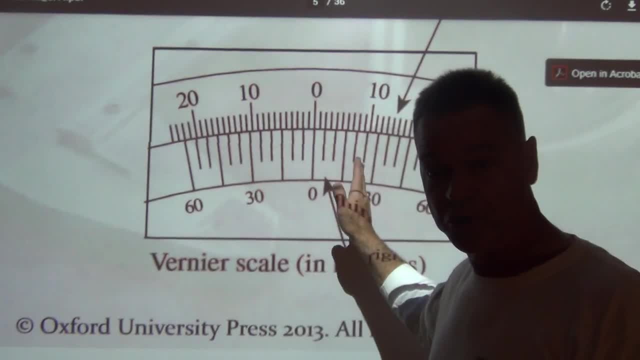 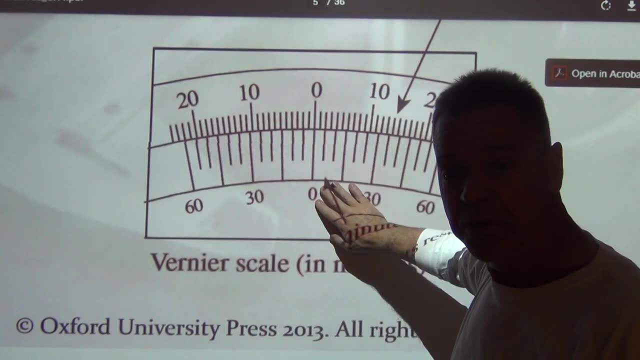 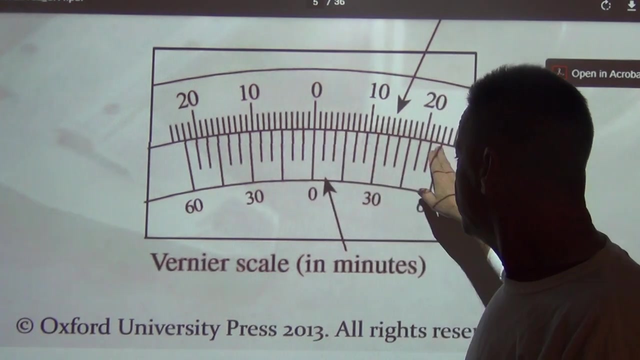 They're not a degree, right, They're actually. in this case they're larger than a degree. They're not 2 degrees. I would say they're just a little bit less than 2 degrees on here. If you can figure out a measurement for these spaces here that makes them just that much smaller than 2 degrees.